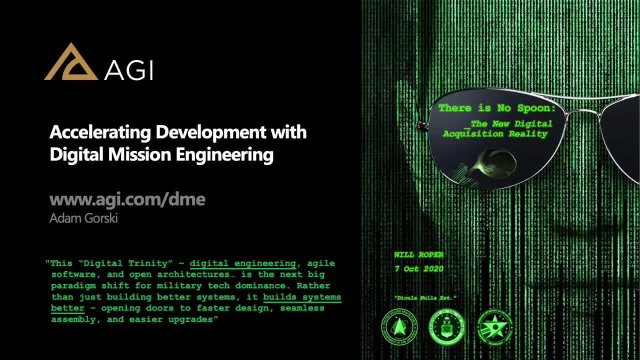 adversaries is forcing a revolutionary change in how we develop systems To meet those challenges. very rapidly, we need to develop some of the most complicated systems ever faster than we've ever developed things, and digital engineering is one of the cornerstones of that strategy. Now there's a lot of confusion about digital engineering. 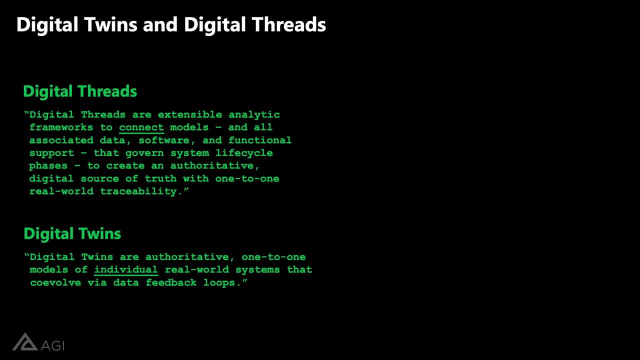 and two of the most commonly confused phrases that I encounter in my career are digital threads and digital twins. We're going to pick this apart a little bit and walk through a real world example of how we can develop systems faster than we've ever developed things. 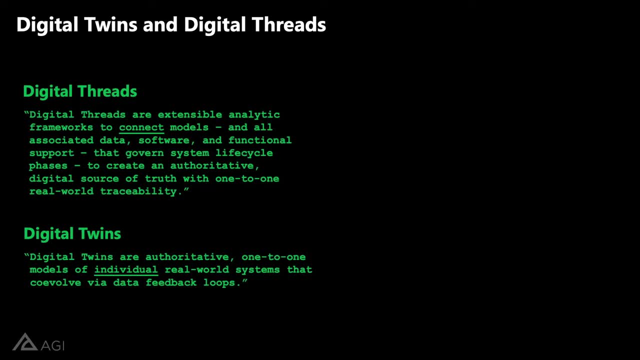 How these can dramatically accelerate the development of a system. Now Dr Roper has provided some really great definitions in the publication. They differ a little bit from the standing definitions in the Defense Acquisition University, but ultimately there's a lot of similarities. So just to get us all on the same page, a digital thread is really this connective. 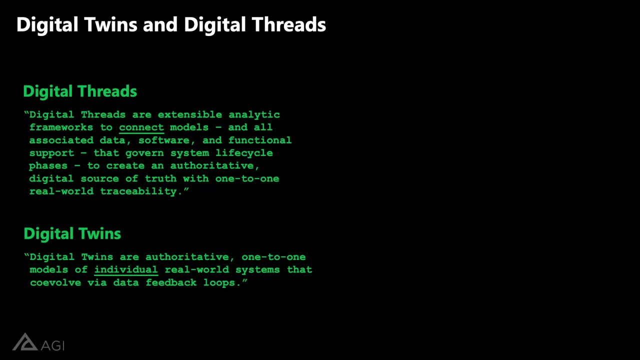 tissue. It's an analytic framework that connects lots and lots of different types of models, software and data- And I'll talk about what those models are in a little bit. but really it's that interconnective nature of all of these disparate descriptions of a system and models of a system. 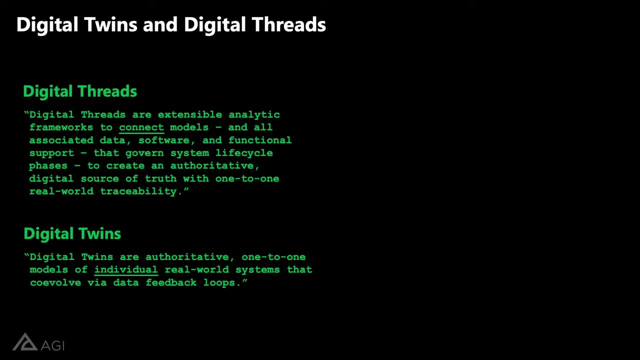 that map to a real world system that's being developed Now, a digital twin. on the other hand, that is literally a one-for-one matchup, a digital version of some physical reality, So for a spacecraft or a constellation of spacecraft or a fleet of aircraft. 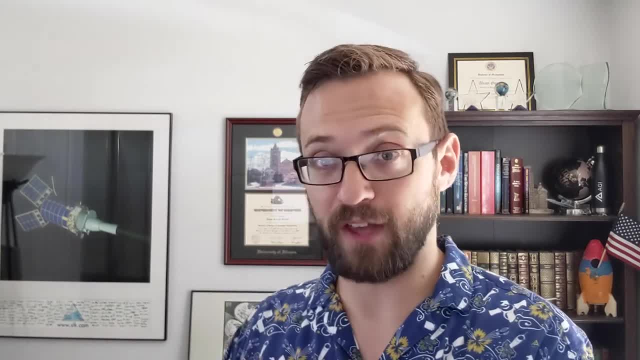 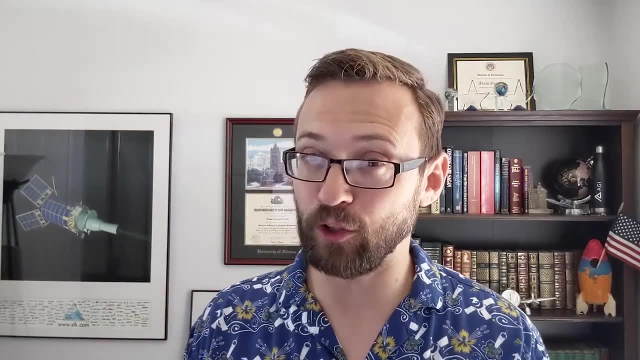 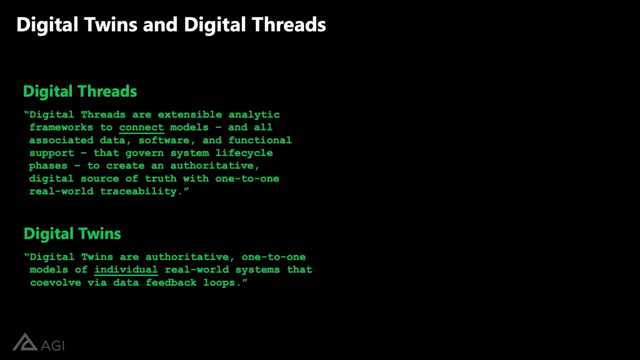 there would be a digital twin of a particular tail number And that's all of the models that represent that particular system that has a constant feedback loop of real data from the real system that's constantly maturing that data. Now, many times that digital twin is built on a. 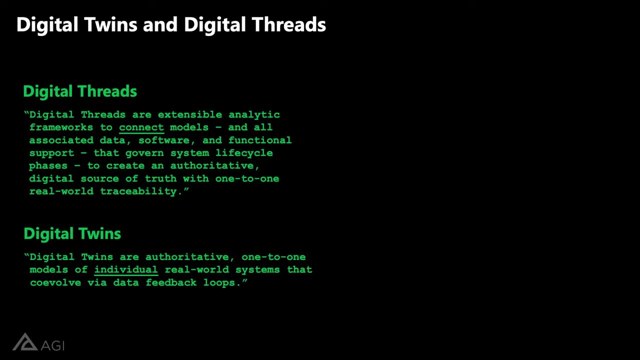 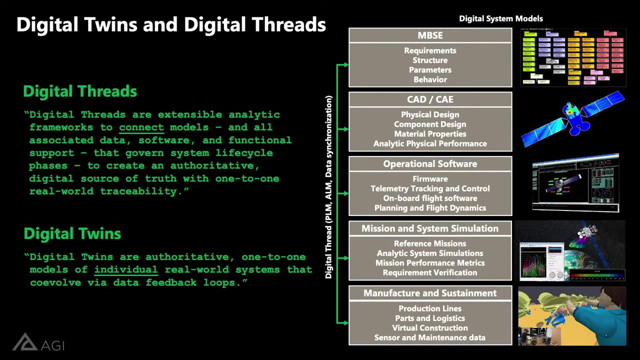 foundation of these digital threads. So these are a little bit different, but let me let me break this down into some real-world examples. There are a lot of different types of models and I think it's important to understand these. So the first type of model that people usually are talking about is a descriptive model. 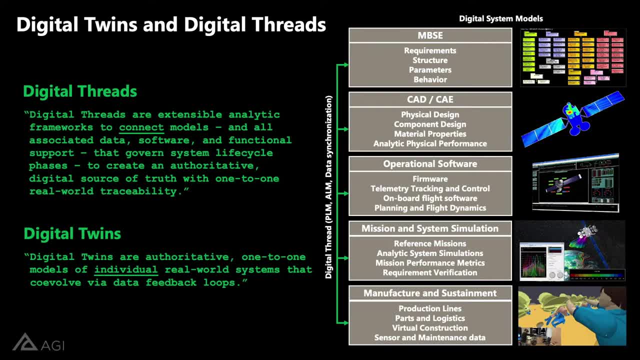 of a system or an architecture. The model based systems, engineering or MBSE models that capture the requirements, define the architecture or the structure, have parameters that define that and also capture the behavior of how the system's supposed to respond. There's also physical models or CAD models that 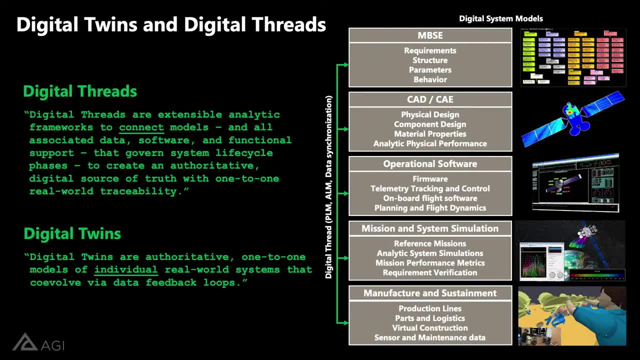 are actually the shape of physical thing that's going to be built And that's usually supported by computer-aided engineering or CAE. Stress and strain and aerodynamics and ray tracing- all those physics models that understand how that physical thing fits together and how it performs in that assembled 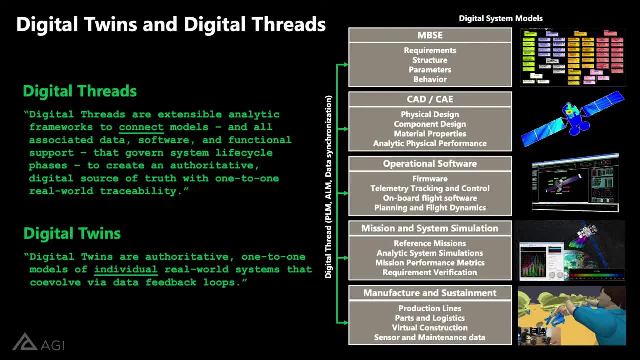 state. Now there's two other types of software that are very common in this. There's the operational software that will actually control an aircraft or a spacecraft: The onboard software, the control individual components. Or, for a spacecraft, you have onboard flight software. 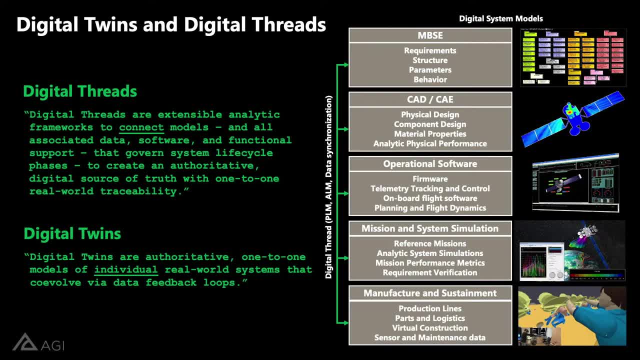 and you have ground systems for flight dynamics and other mission planning and scheduling. Those are very common. Now, another type of software that is always present in the development of these systems is this fourth block of mission and system simulation. These are often called analytic models, because these analyze and evaluate the performance of the system as it's. 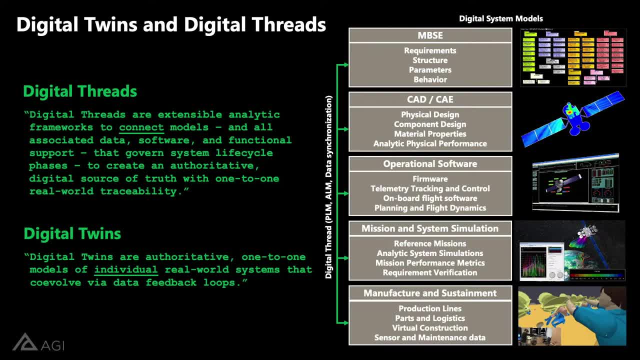 designed. The system that I'm designing, will it meet the requirements that I've defined my system's supposed to meet? This is arguably one of the most critical parts, because this is where I start verifying that the system I'm designing will meet the requirements I'm asking it to, And this gets. 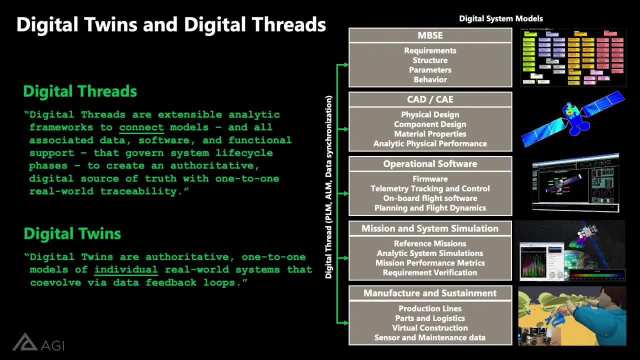 revisited at every stage of the life cycle to make sure that the system can perform as expected. And finally, in a digital thread and in digital twins, there are often simulations of the production In a digital reality construction and, most importantly, in a digital twin. that real 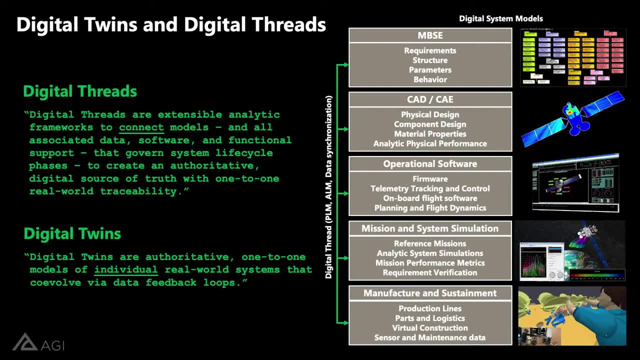 feedback loop of sensor data and maintenance data under sustainment. that's evolving and maturing that model. Now at AGI we're not going to pretend we do all of these things. We understand that the digital thread has lots of different commercial parts of PLM and ALM and data synchronization. 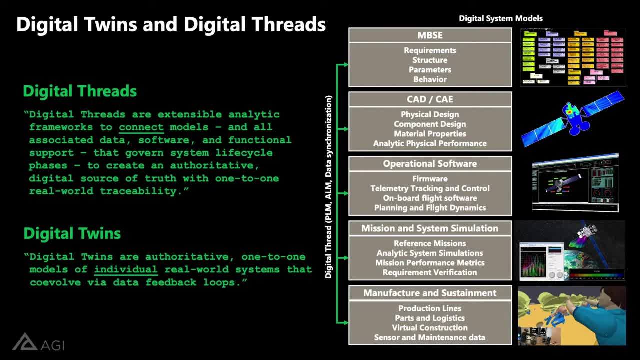 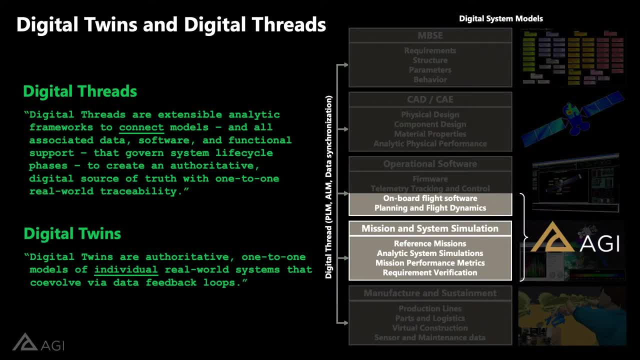 and orchestration pieces, But in our 30 years we've focused and have extensive experience in the operational software that controls vehicles and flies vehicles, as well as those analytical simulations that validate mission performance and system performance. And this is a really key part of model based verification, so that you can rapidly start. 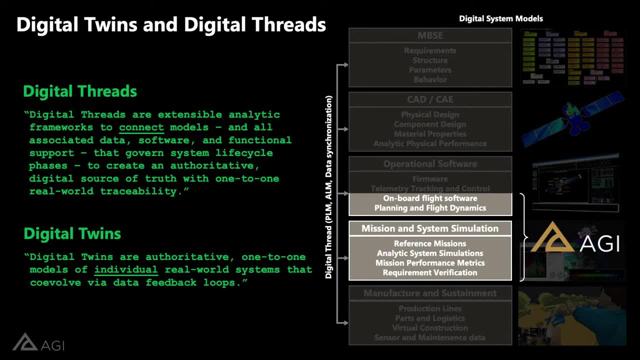 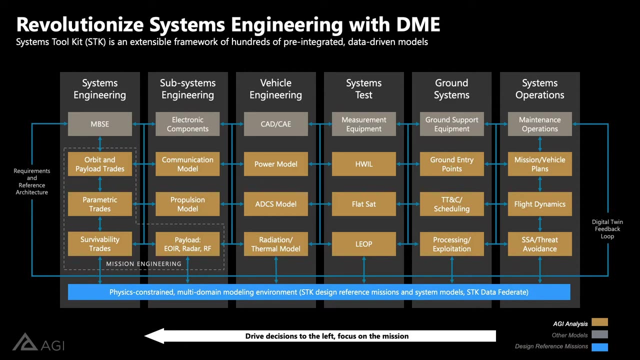 testing a system earlier in the design life cycle, before you start bending metal and flying it sooner. So let me break this apart in a real world example. Most organizations that we've worked with, and we've worked with thousands of different programs and hundreds of companies around the world really, and there is usually this: 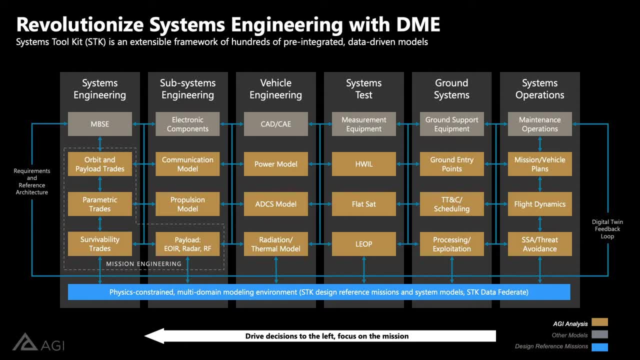 matrixed organization and these systems are enormously complex and they require specialization. You have systems engineering, subsystems engineering, vehicle engineering. for the structures You have whole teams dedicated to testing the system. You have ground systems to control and fly. You have folks specializing in developing those systems and teams that train and operate. 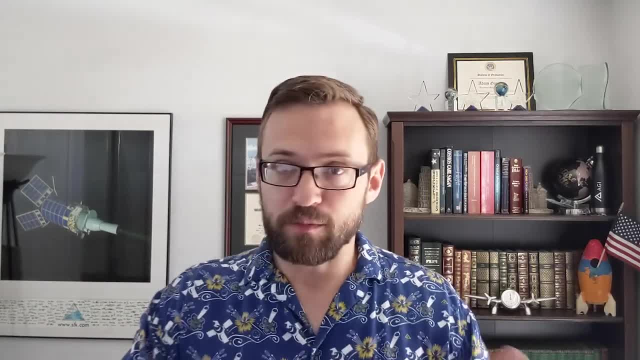 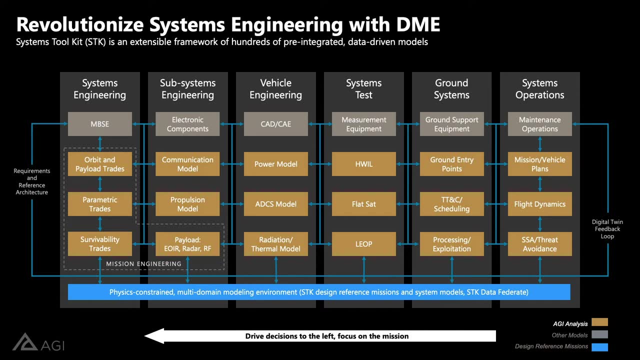 those systems. So these are common and your organization may look a little different, but these are common breakdowns of silos that often exist within organizations And we've talked in other AGI presentations about how these disparate organizations and the replication of models across these silos can lead to extensive reinvention In the context of a digital twin, the US. 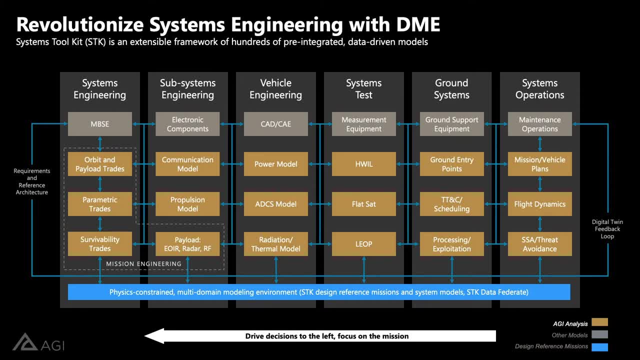 Air Force and the Stevens Institute of Technology actually performed a Kokomo trade study to evaluate the development of a digital thread and a digital twin, And there were some flaws in the study. I've read it. It's good, But they came to the conclusion that developing 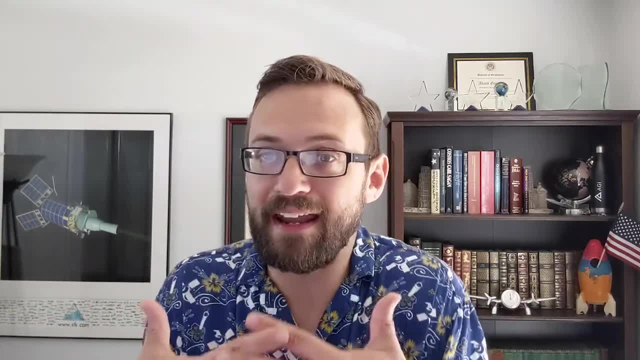 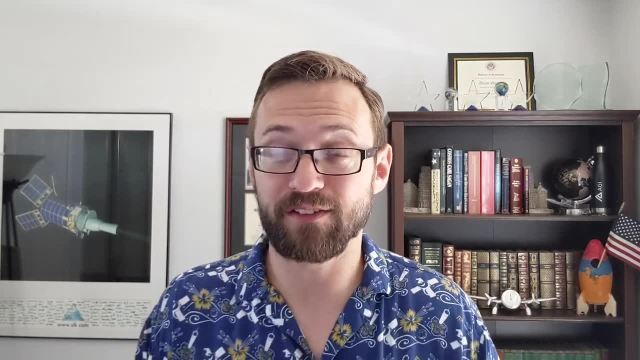 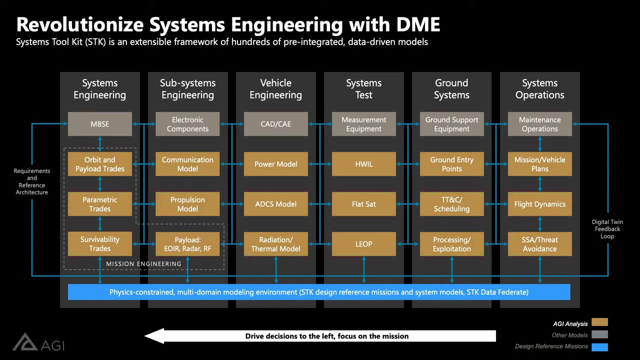 all of these models and developing all of the interconnective tissue of a digital thread could cost billions of dollars, Billions of dollars, And fielding these models and developing a fully functional, completely integrated woven digital thread could cost hundreds of billions of dollars, just on the amount of software code it would take to write all these. 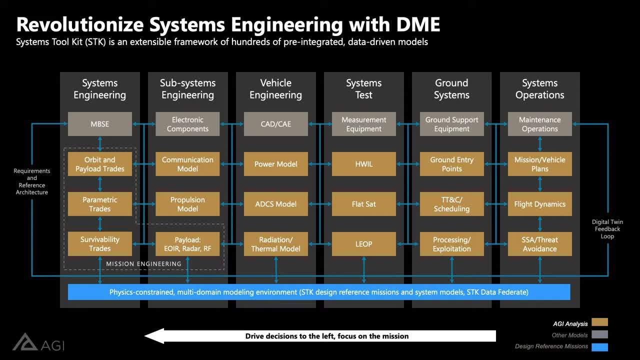 models and stitch them all together. Again, I believe that there are some errors in that, but the fundamental takeaway is: this could get really complicated And today the way most things happen are we have these well orchestrated organizations where systems engineering will do a trade study. Let's talk about a. 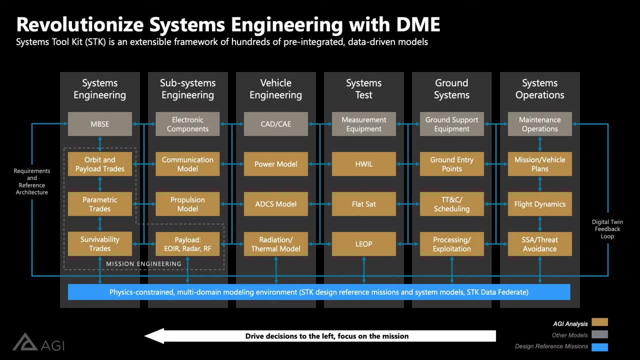 space system. They'll do an orbit trade and start figuring out the orbits that meet certain requirements And then they'll generate, typically in that left side of this diagram, in mission engineering, a design reference mission And the point of that will be to find critical. 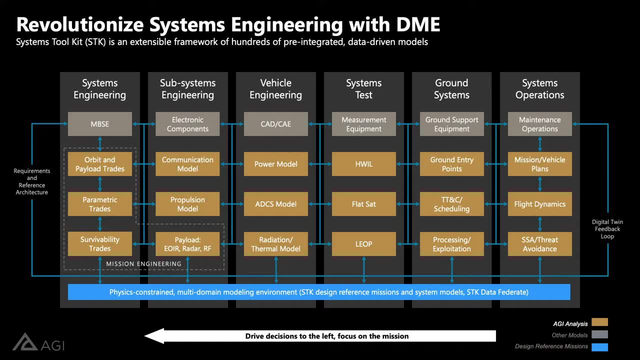 corner cases or critical data. for how much time is that spacecraft in the sun? What are my ranges as I overfly my ground stations? And they pass that data to other teams, Then the computer will be able to do that, And then the computer will be able to do that. 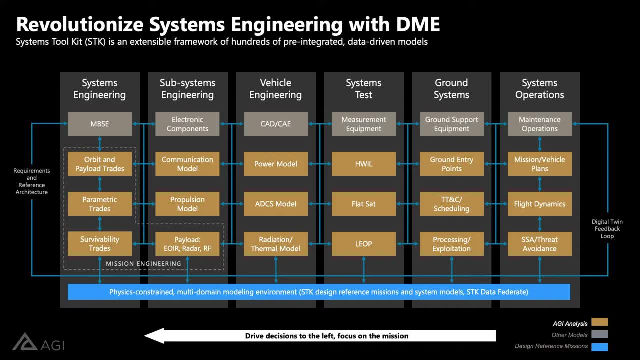 The communications team takes that for instance and they put it into their own model of communications to then design a communication system and verify that they'll be able to communicate with those ranges and contact times. They'll take those sunlight times and pass them to. 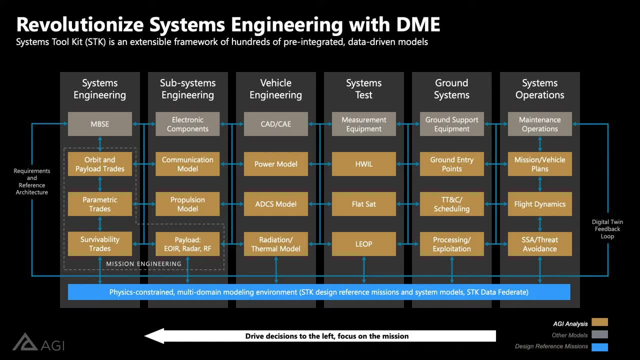 the power team and they'll have to verify that they can meet their power budget. But now the radiation team starts understanding and they're saying: well, you know, we need some additional shielding, We need so that adds mass. Then that changes the orbit that they can reach. Now they change the orbit, Now the 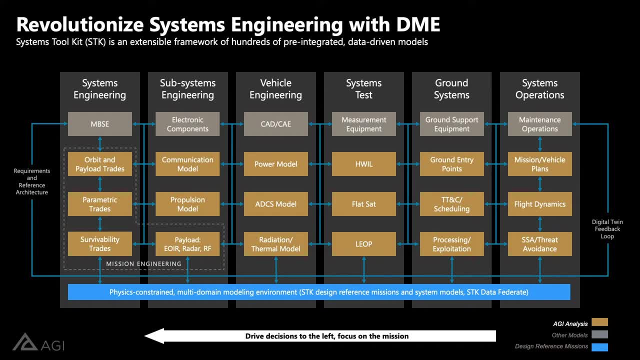 communication team needs to reevaluate their communications link And the power team needs to reevaluate their power analysis And that type of passing information that gets manually put into a new model and oftentimes in every program these models get built over and over and over again. that happens countless times, hundreds of times on most large programs. 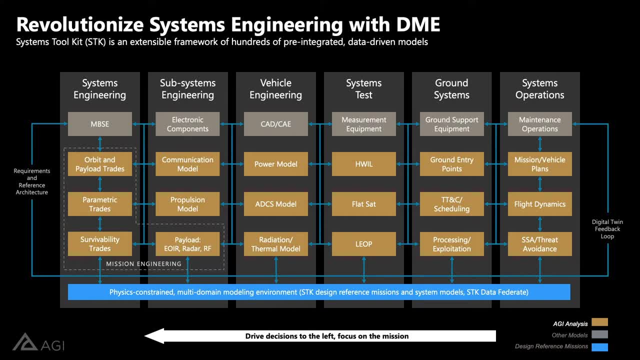 constantly reinventing models, constantly manually passing data and storing all of this data. The promise of digital mission engineering is when I can integrate those models, then when I make a parametric trade where I've optimized against an orbital altitude or an inclination that can ripple through my other models And I can instantly verify that that 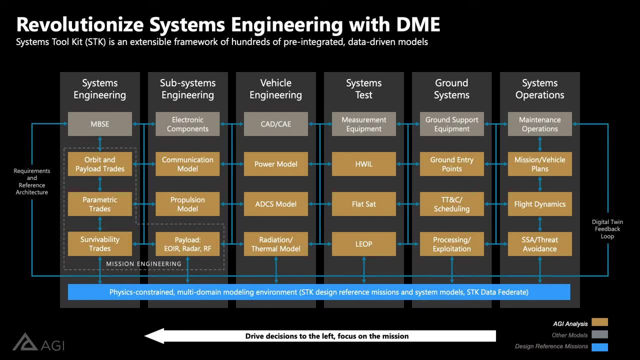 design reference mission. as designed, Can it still meet my link budget requirement as the communication model is designed And I can instantly verify that requirement without having to manually go and redo all that I can. I can get instant model-based verification of my requirements. 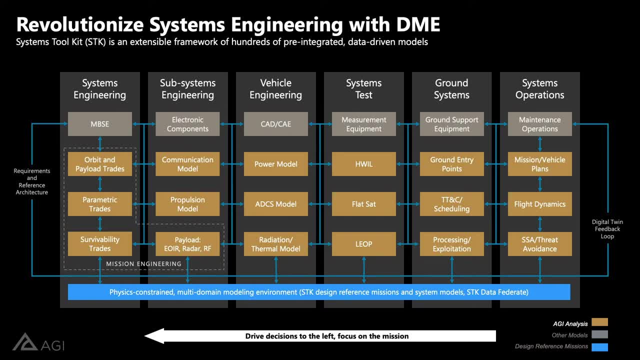 And as many times as this happens, this can dramatically accelerate a program. Now it's interesting: at AGI we make Systems Toolkit, which is, by definition, an extensible framework of hundreds of models. It's a very complex framework. It's a very complex framework. It's a very complex framework. 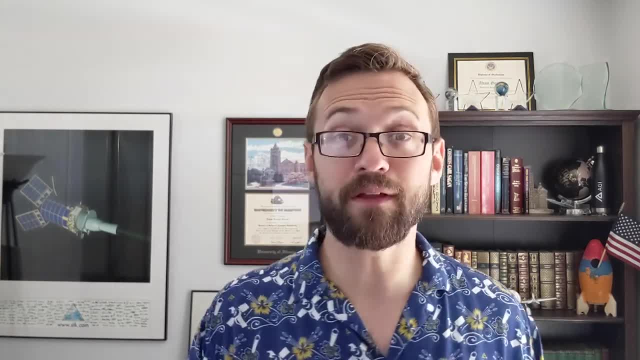 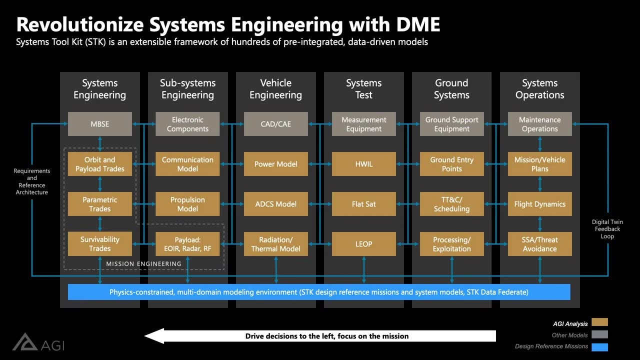 There are hundreds and hundreds and hundreds of pre-integrated and data-driven models. That means they're driven by data or they're driven by parameters that can be natively linked within a model-based systems engineering model. We're going to walk through each of these very quickly. 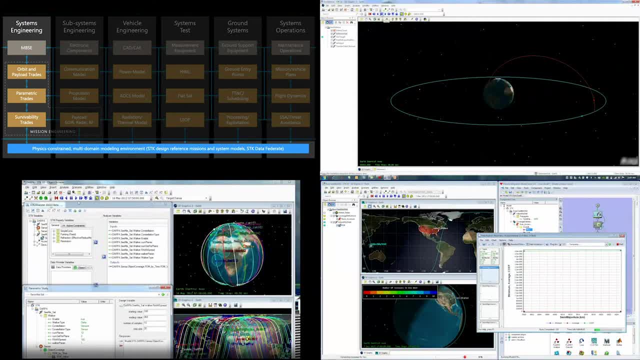 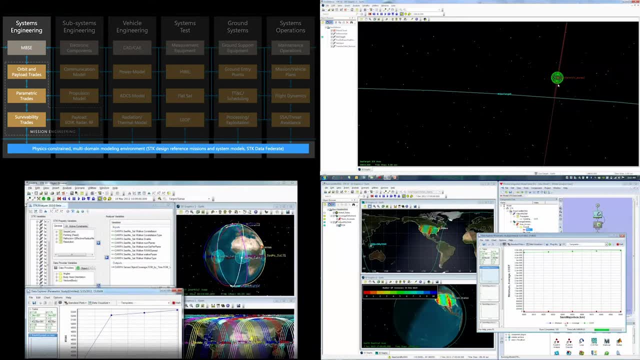 Most people know of AGI for orbit and payload trades- that early kind of analysis where I start understanding my orbit analysis. But in addition to that we have a multivariable optimization environment for parametric trades that allows you to take those orbits and other. 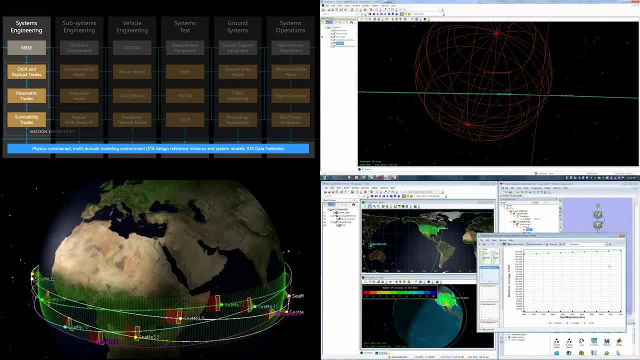 parameters and start analyzing them. We're going to walk through each of these very quickly. Most people know of AGI for orbit and payload trades. that allows you to take those orbits and other parameters and start doing a multidisciplinary analysis and optimization, an MDAO. 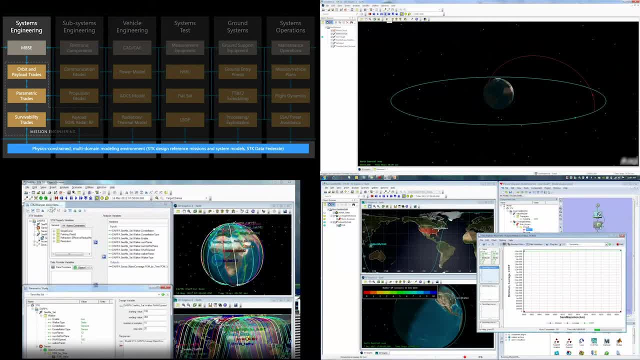 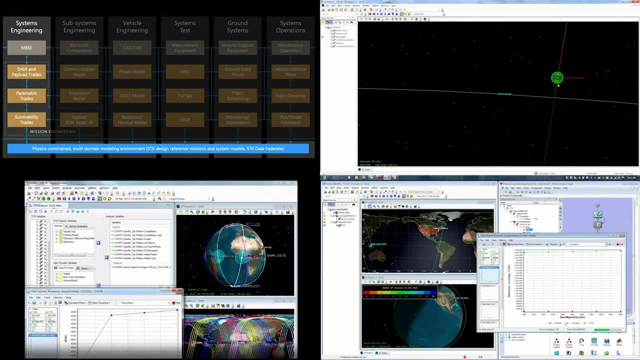 Survivability trades, as you see in the upper right corner of this video, looking at the reality that we have threats, we have a crowded space environment, we have adversaries and the ability to study your spacecraft's ability to survive those engagements, to have defensive 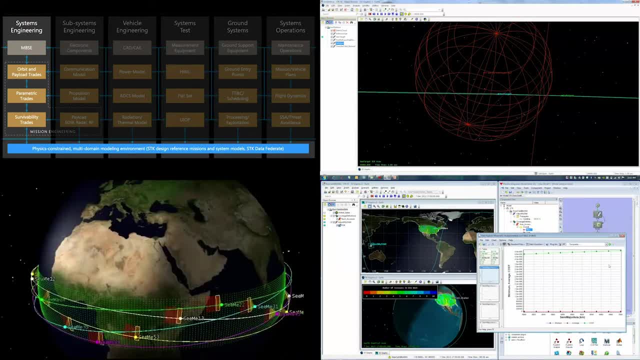 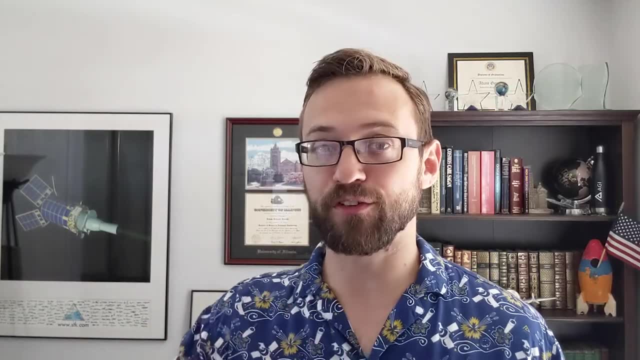 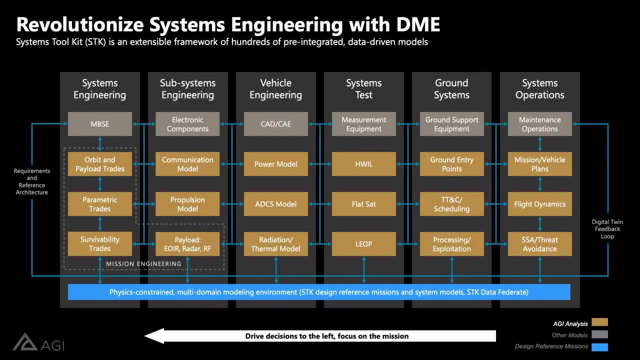 countermeasures. Those are things that people study with our software. What's interesting is every gold block that you see on this diagram. Someone in the industry has done a build versus buy of leveraging AGI's software to perform that analysis using these models. 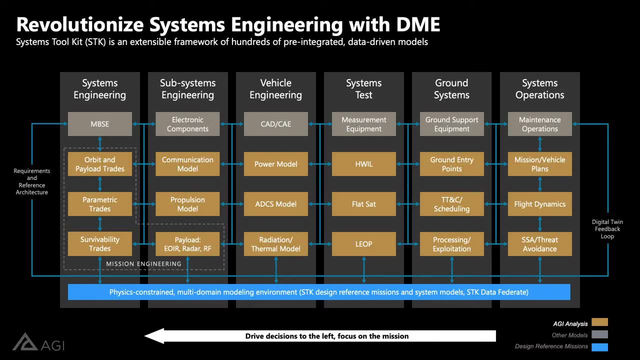 So every block. someone has completely justified their entire investment in AGI software just to satisfy one of these blocks, usually in a silo and in a stovepipe, completely disintegrated from all of the other parts. As more and more parts of an organization have been destroyed, they've been completely 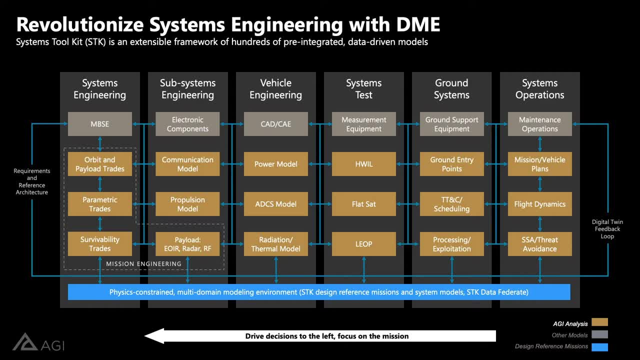 disintegrated from all of the other parts. As more and more parts of an organization have been destroyed, they've been completely destroyed, And so we need to do a bunch of other things in order to get a better understanding of what that looks like. 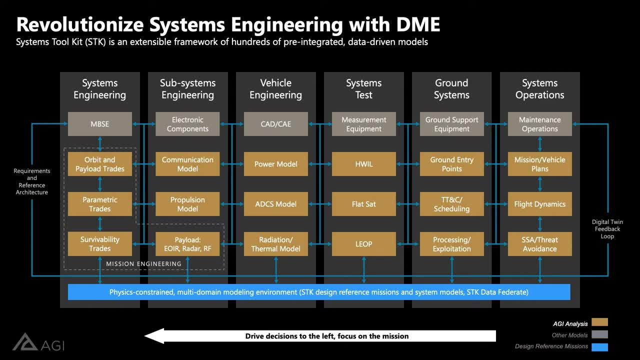 So yeah, I've talked about this a lot. It's a great question. It's a really interesting one. Definitely we've talked about this a lot. actually, You know, as an organization I've talked about it quite a bit on this panel. but this 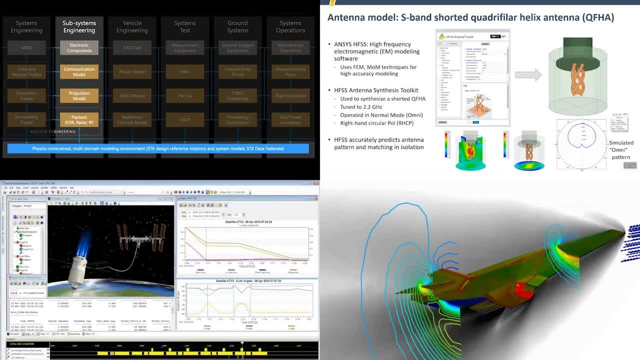 one is a little bit more interesting, but it's very good. It's a great line to start. I'm not sure if anyone can get that, But I'm not sure if anybody can get it right, but it's really great. That is a great question, but it opens the door for me to think about it a little bit. 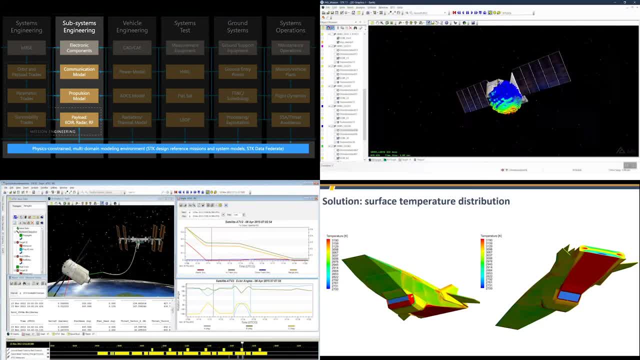 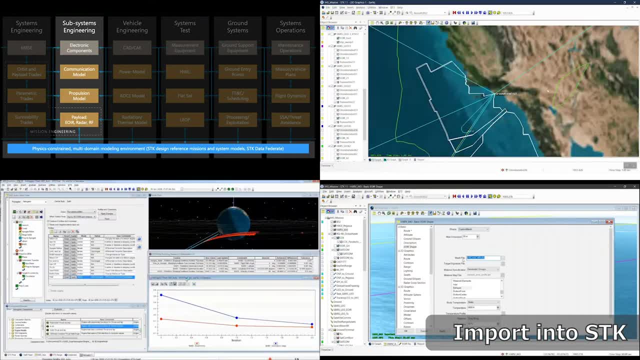 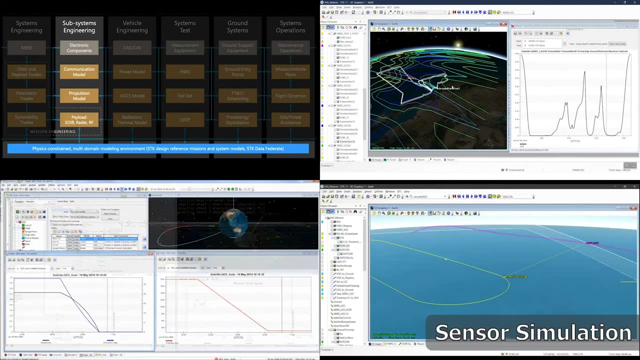 What it means is you can take AGI software, steel blocks, a couple of units that you're going to create with a small cloud cluster. Yeah, design reference mission And SDK provides dozens of pre-installed communication models for antennas and ITU standard propagation models. You can also supplement that with as-installed CAE data. So 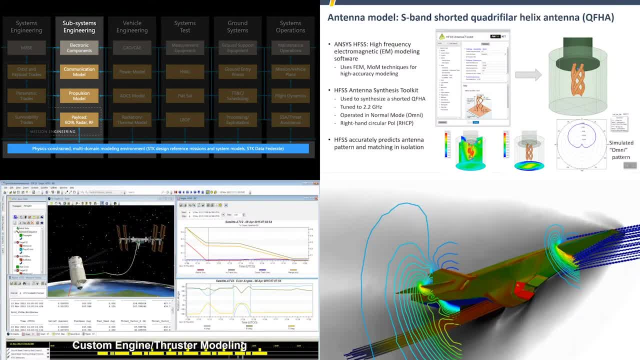 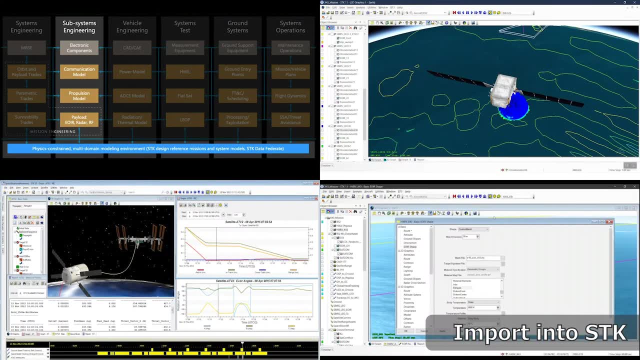 again. I've got anechoic chamber data or simulated ray tracing of that antenna installed at that point. What is the far-field radiation pattern? What signal strength is going to get down to my ground station? That model is completely available inside of this environment. The propulsion model. 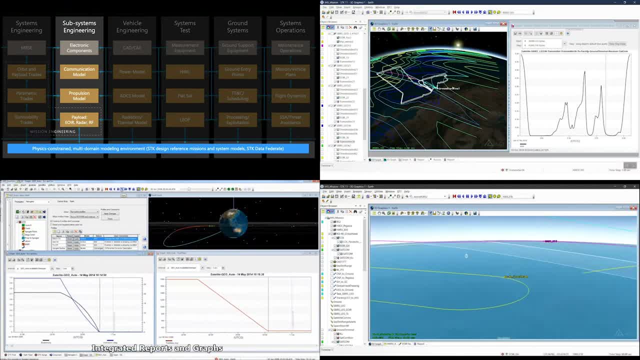 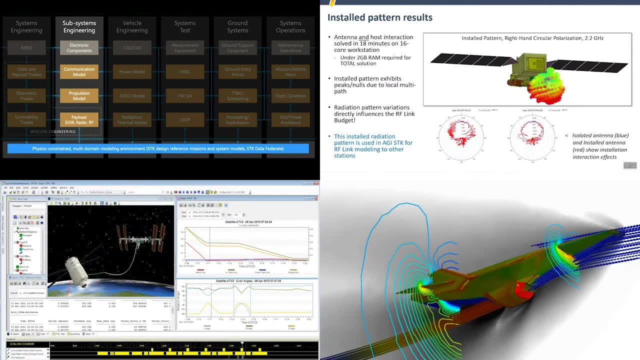 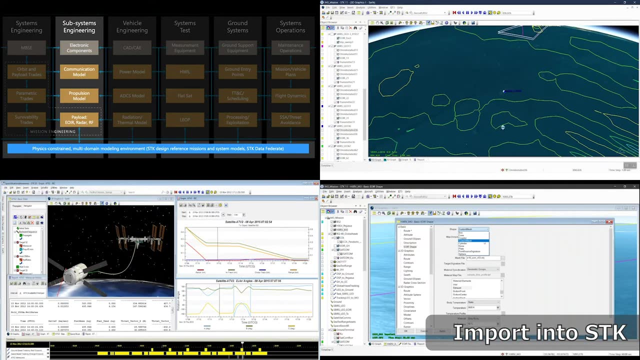 for evaluating delta V studies and lifetime station keeping or rendezvous and proximity operations. We have customers. the Space Dynamics Laboratory has completely validated and verified our EOIR, electro-optic and infrared payload modeling, our communications modeling, our radar modeling. Those are models that are common subsystems, that are fully vetted and integrated. 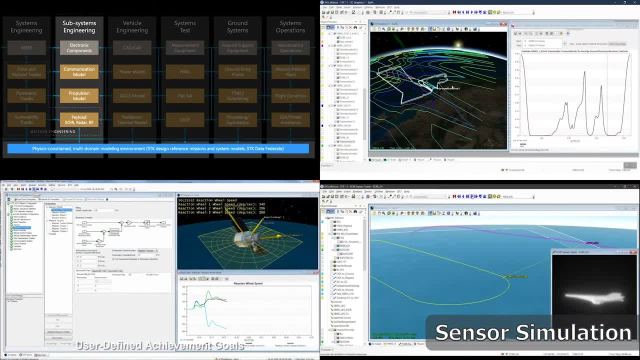 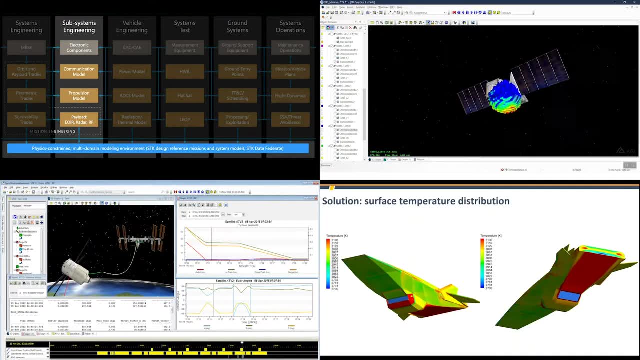 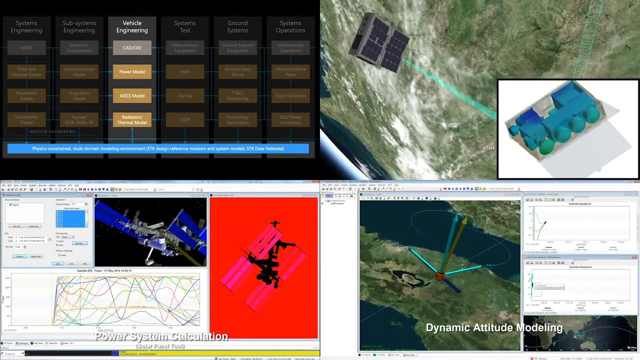 into this environment For very detailed analysis. So what would that particular hypersonic vehicle look like with this sensor, with these parameters? And as I do my trades, I can start to evaluate that. And then, as I move in over to vehicle engineering now, I take those CAD models and other data and I can feed that into. 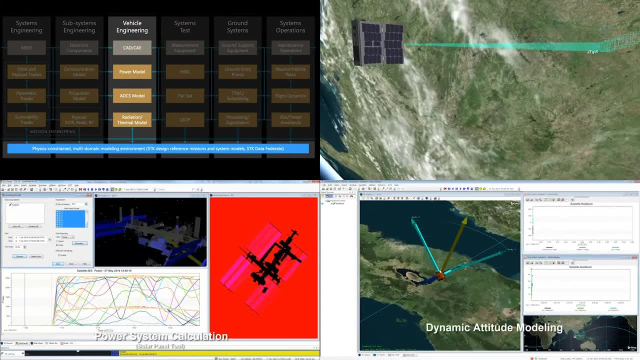 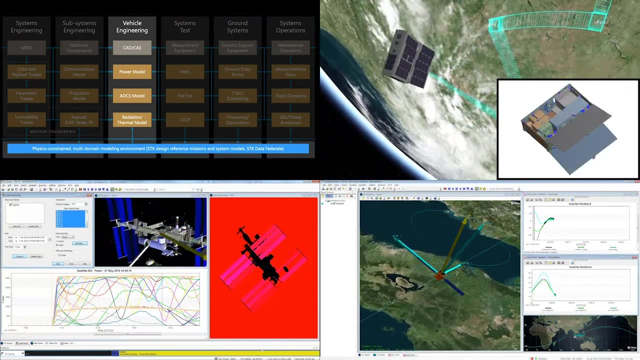 the power model. In fact, the International Space Station, the largest structure on orbit, uses STK for their power model. Because of the fidelity with which we can use STK. we can use STK for our data. We can take the structural dynamics of how that system is moving and the shadowing of the solar 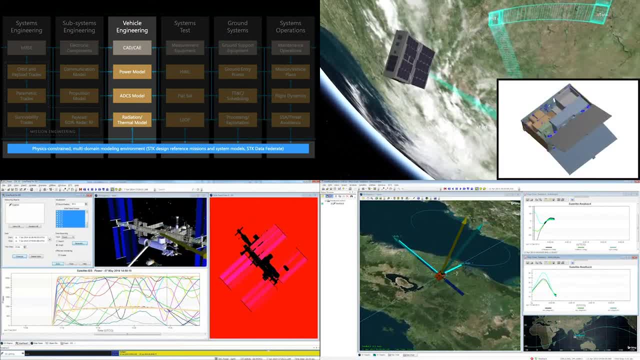 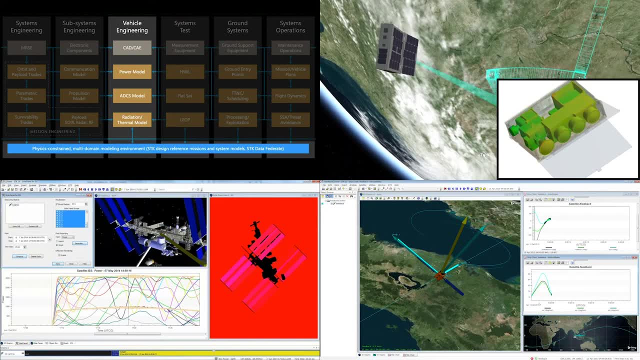 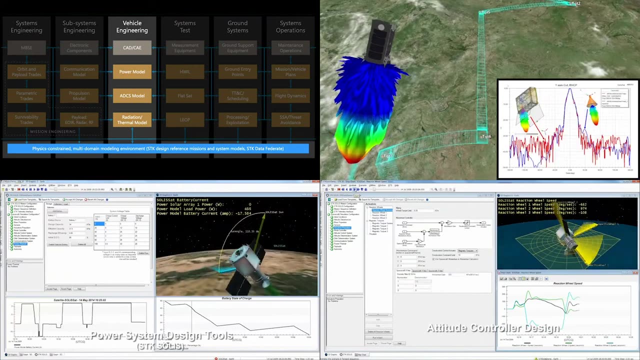 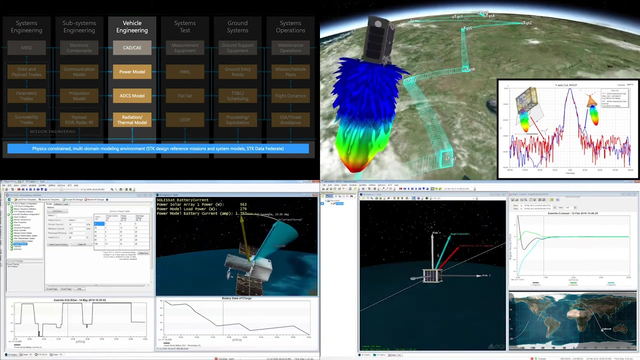 panels on the other solar panels. All of that can come into account. That used to take NASA weeks and weeks to just analyze a few orbits worth of data And now they can do that in hours. And it's incredible the fidelity that's afforded here For the ADCS, the Attitude Determination and Control System. inside of this framework there is fully vetted flight. 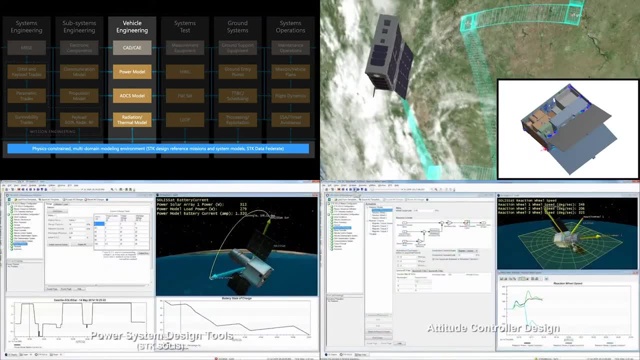 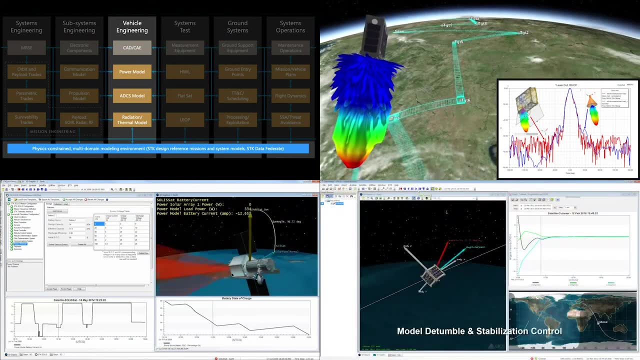 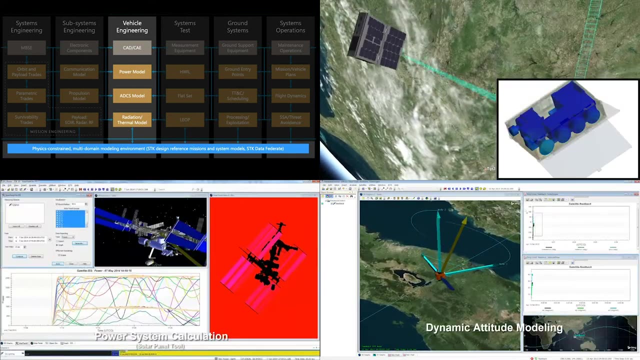 software that is currently flying on about thirty different satellites. some haven't launched yet, But actual flight software fully emulated inside of this environment, so that I can understand when I'm doing my reaction wheel sizing and doing these other things. I can understand how the system is going to react to those changes. The radiation and thermal environments are integrated. 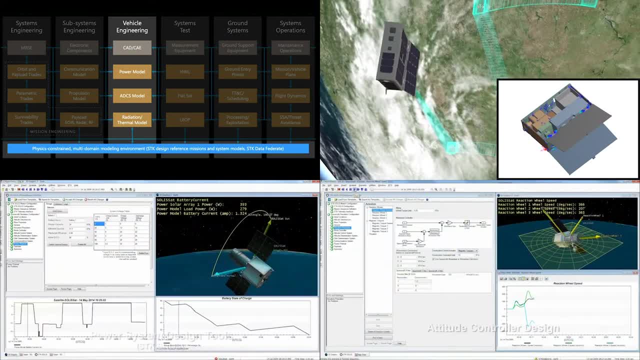 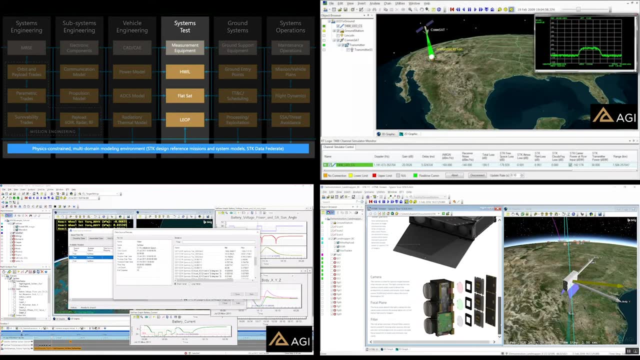 inside of this environment as well, so I can understand my radiation dose as I change my orbital parameters- Again all pre-integrated, When I move into systems test. you can start moving into system test almost on day one, because now I keep maturing these models and I'm constantly testing them. 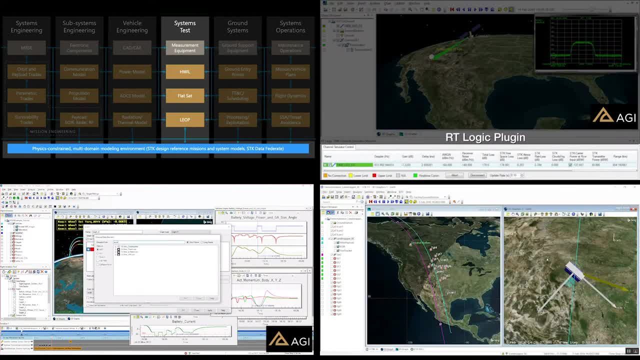 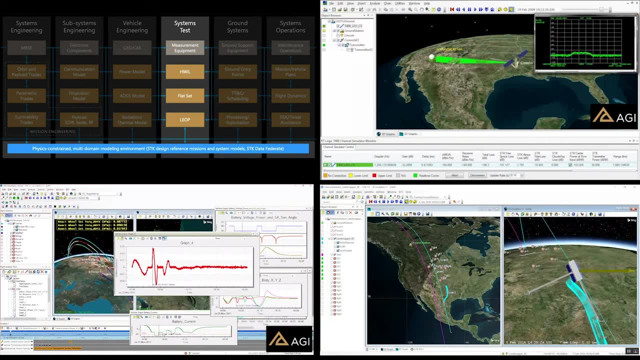 As the system design matures. now I can start getting hardware and plugging it in. get hardware in the loop. Customers do this all the time because the data coming out of the SDK models is so realistic It's indistinguishable from a real world signal. so I can plug it into hardware in a loop to 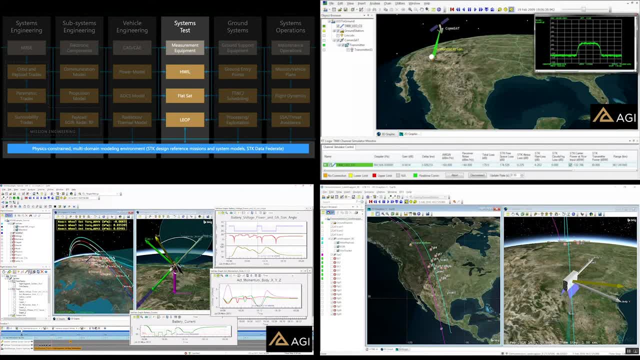 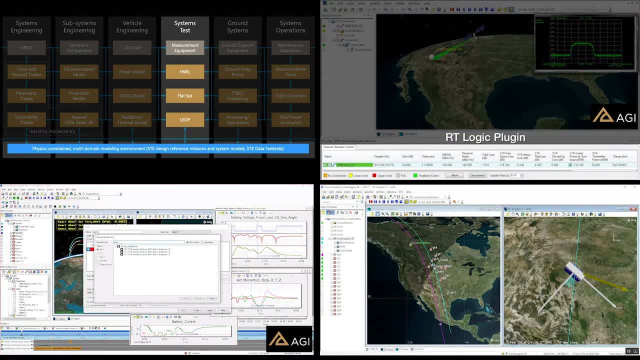 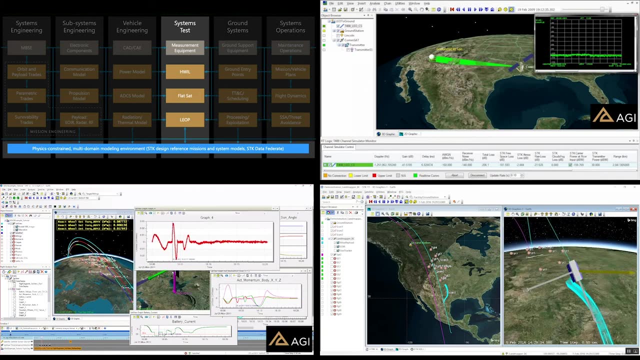 understand how that hardware is going to respond. I can have that virtual flat sat where I can test my commands. I can understand how is the spacecraft with that ADCS model going to respond to these commands. so I can start testing this As I move into actual launch and operations. all of these really powerful workflows for 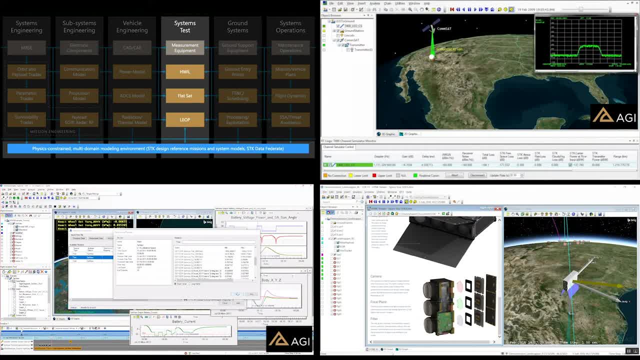 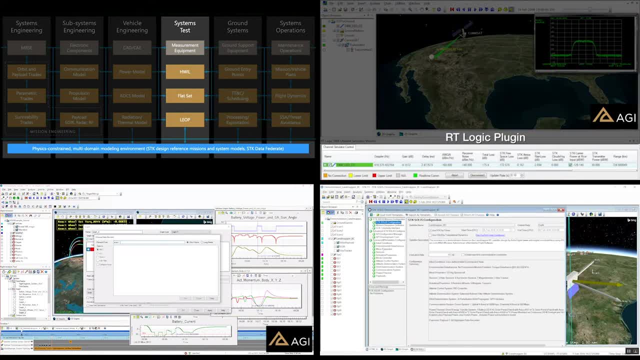 taking that sensor data, the real telemetry data, the real sensor data off of the spacecraft and comparing it to the model. as you see down there in the lower left, all of these tools for verifying performance And updating the model are readily available, so now it just becomes a matter of updating. 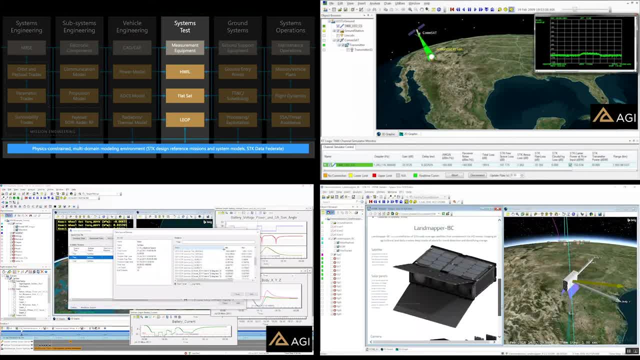 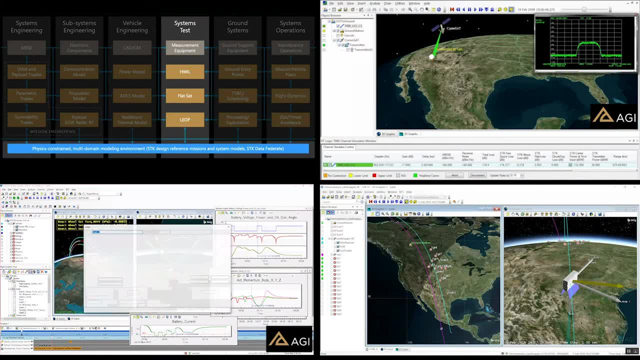 the parameters- Hey, that thruster is firing a little hot or hey, this reaction wheel rate is a little bit off. That can get fed back in and so future planning can take advantage of that. And the goal is that now, when I move into my ground systems and systems operations, 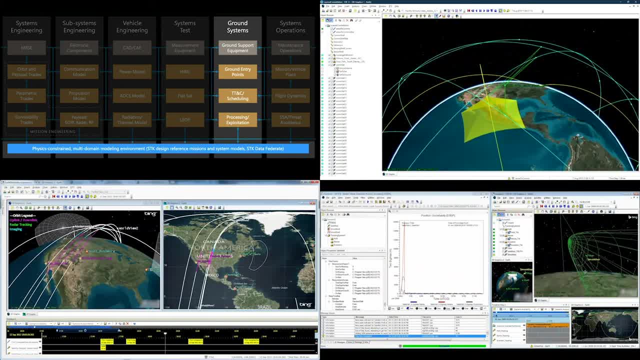 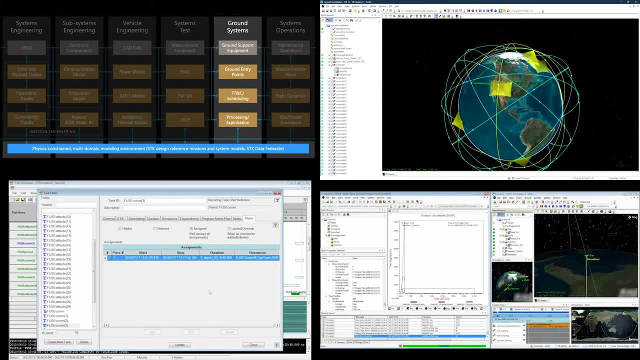 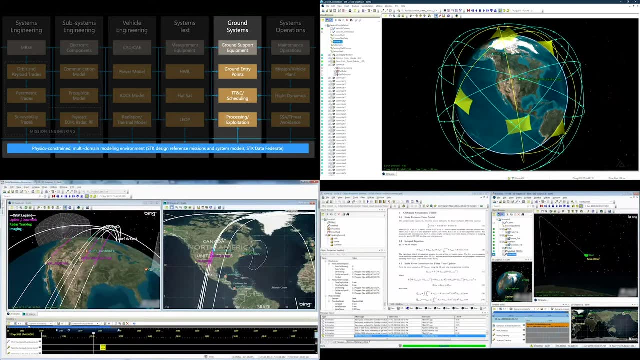 not only can I design my ground systems, I can design how many ground sites I'm going to need for this large constellation, accounting for all the real world conditions. I can actually start embedding this digital model and this technology into that ground system. These are open programming interfaces, application programming interfaces, so you can plug these. 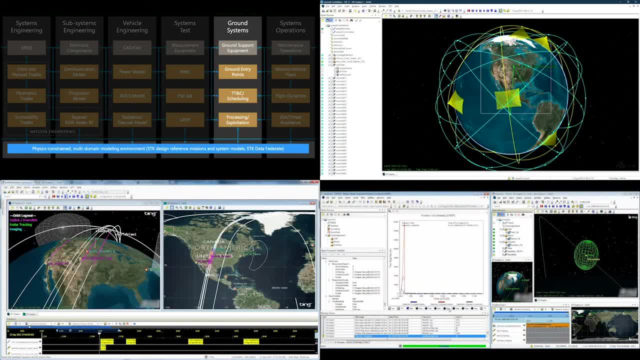 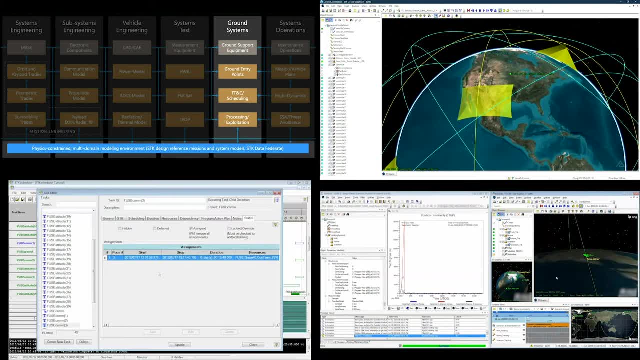 models directly in, and, as your model matures, you now know how it's going to operate. We have extremely powerful scheduling algorithms that are completely built, that take into account everything that we've just talked about, So now my scheduling can account for all of these things. 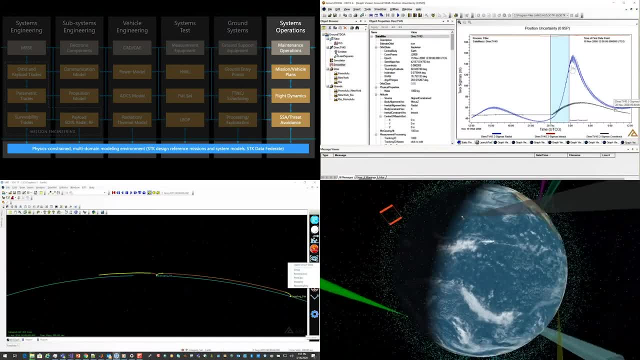 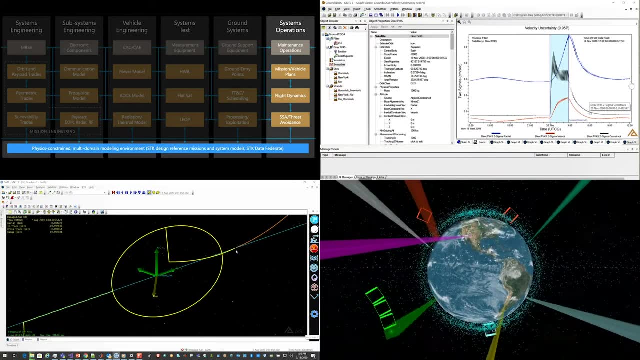 As I move into systems operations. my flight dynamic systems can be built with the plans and the systems And the schedules and the maneuvers that are required to meet these requirements. Some of the most exquisite spacecraft on orbit build their flight dynamic systems on AGI. 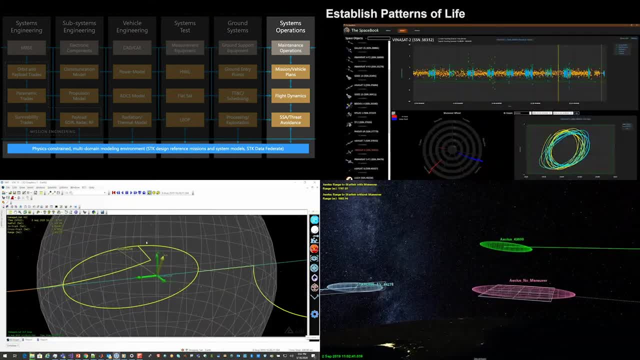 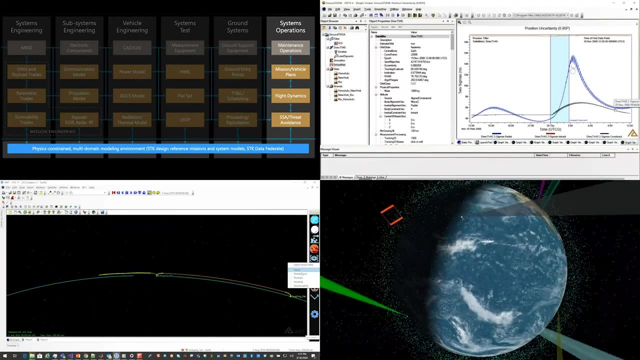 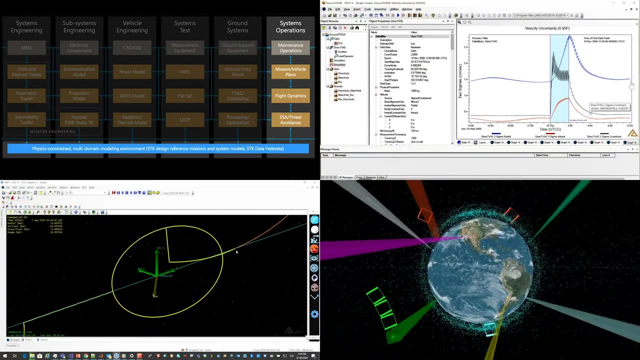 software because it has all of these models, For instance, the TDRS satellites that NASA flies, extremely tight flight dynamics requirements met by AGI software, The Cygnus spacecraft that performs rendezvous and proximity operations with the International Space Station. Some of the most complicated things in space are powered by AGI.